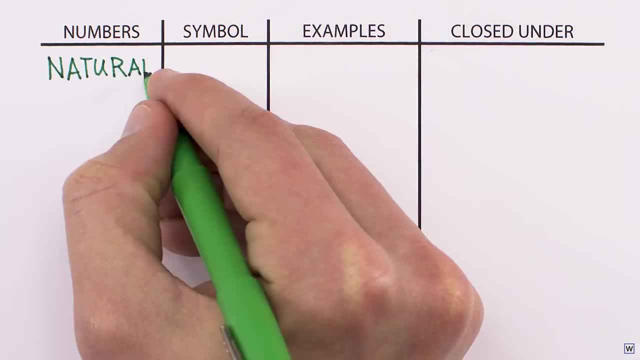 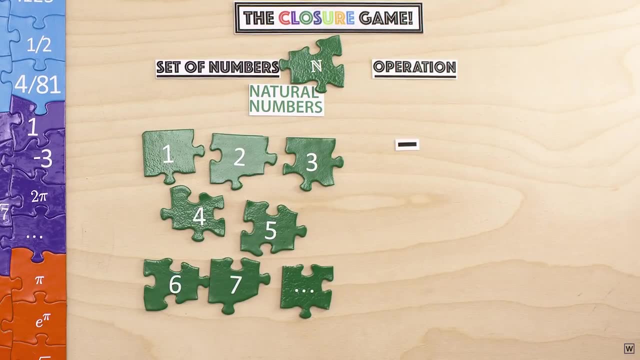 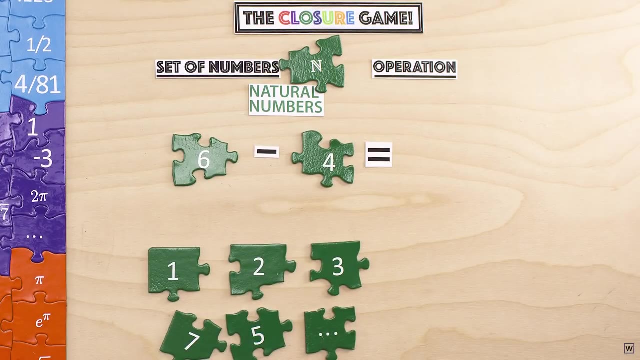 together result in another natural number. Mathematically we can say that the set of natural numbers is closed under addition. Next let's try the set of natural numbers and the operation of subtraction. For some pairs of natural numbers, like 6 and 4,, things work out just fine. 6-4 is 2,. 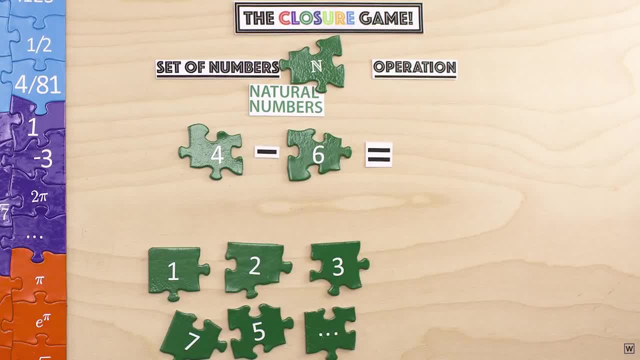 which is a natural number, But what about 4-6?? This results in an answer that is nowhere to be found in our set of natural numbers, so our set is not closed under subtraction. We need to expand our set to include 0 and negative numbers for this to be the case. 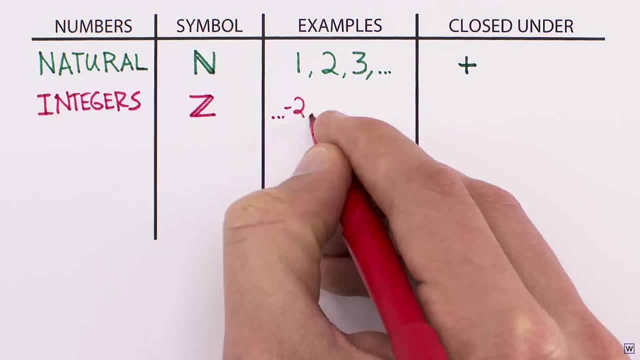 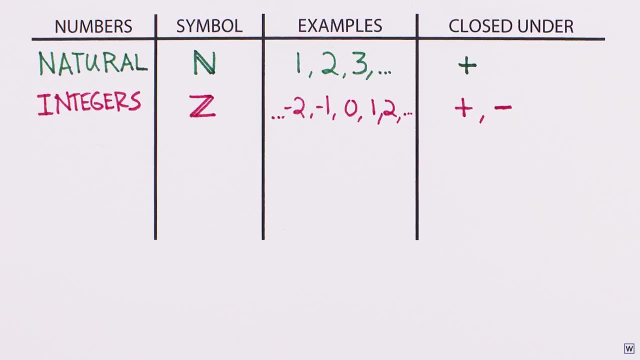 So the set of natural numbers is not closed under subtraction, but the set of integers is. By expanding our number system we can guarantee that any subtraction question we can ask will have an answer. As we include more algebraic operations, we must continue to expand our 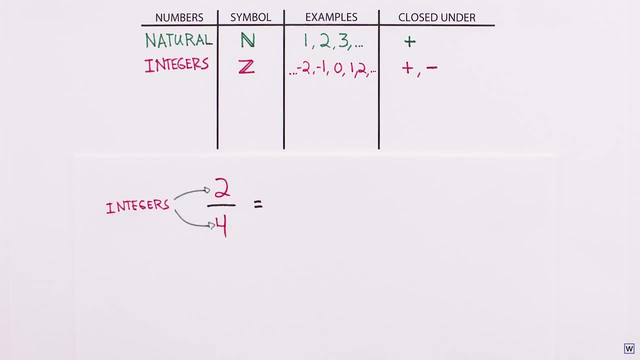 number system. Division requires us to expand our number system to include fractions, also known as rational numbers. Rational comes from the word ratio. Rational numbers are numbers that can be expressed as the ratio of two integers. Venn diagrams are pretty useful here because they help us visually express the idea that 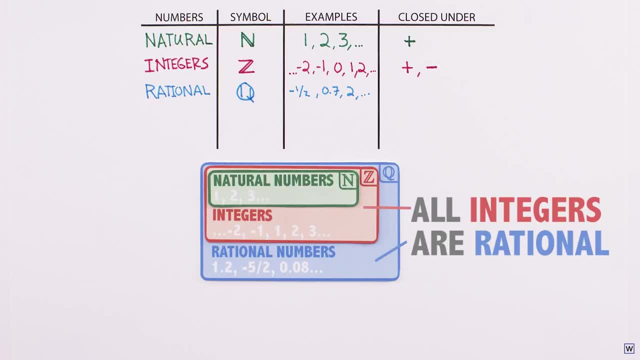 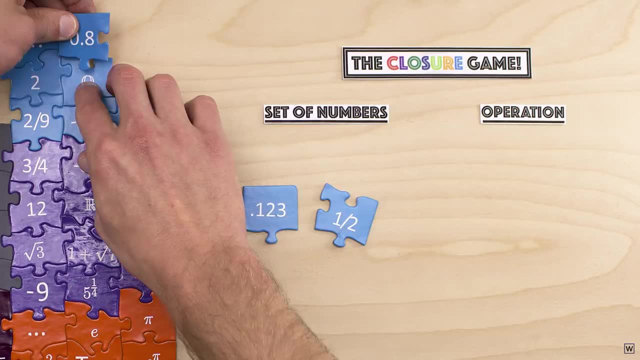 one set includes another. All integers are rational numbers because we can always express them as a ratio of two integers, but not all rational numbers are integers. Let's recap: So far we've made it to the set of rational numbers, which includes numbers like 1, 0,. 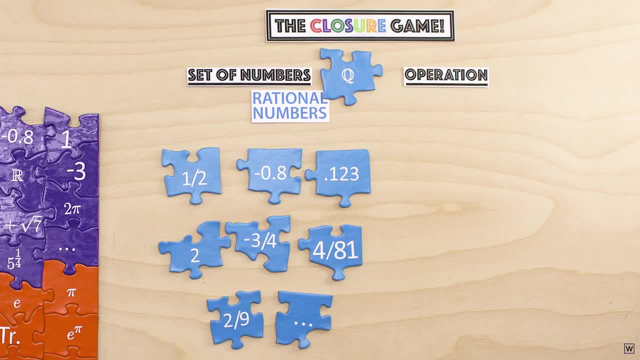 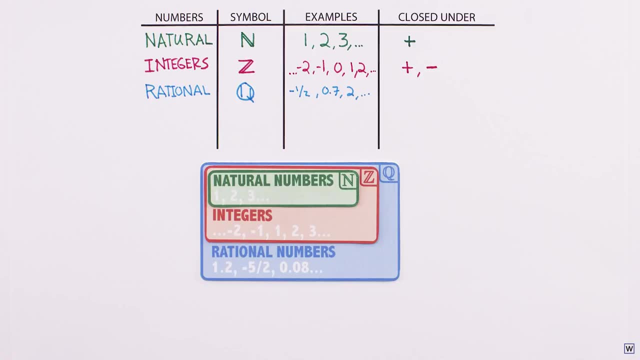 minus 5, and minus 2 thirds. What operations are the rational numbers closed under? Well, any two rational numbers added together yield another rational number, so we can say that the rational numbers are closed under addition. We can say the same for subtraction. 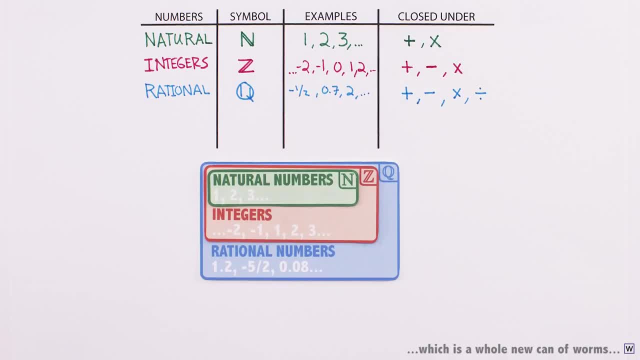 multiplication and division. Now what about powers and roots? Does a rational number raised to a rational power always yield a rational result? It turns out that for problems like 2 ninths to the power of 2, this is no problem. Our 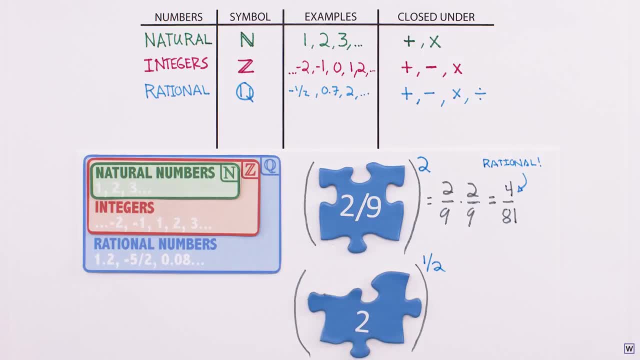 result is rational. Where we get into trouble are problems like 2 to the power of 1 half. Raising something to the power of 1 half is the same thing as taking the square root, so this is equivalent to the square root of 2.. We'll save the full argument for another. 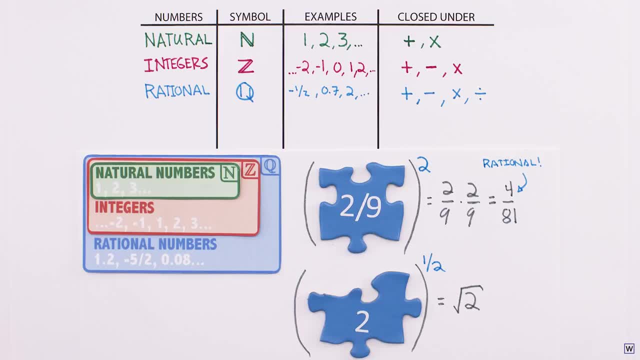 day. but it turns out that root 2 is not rational. There are no two integers that, when divided, equal exactly the square root of 2.. Since numbers like this are not rational, we give them the name irrational. There's one more class of numbers that are even cooler than irrationals: the transcendental. 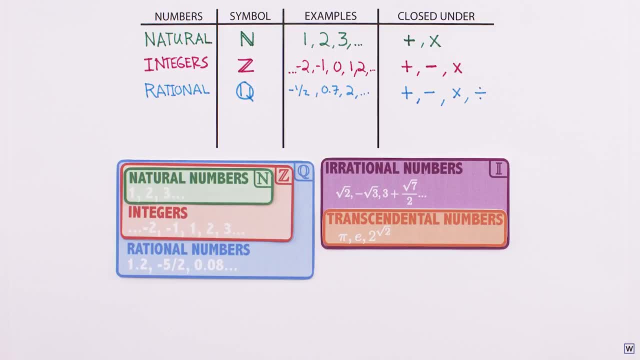 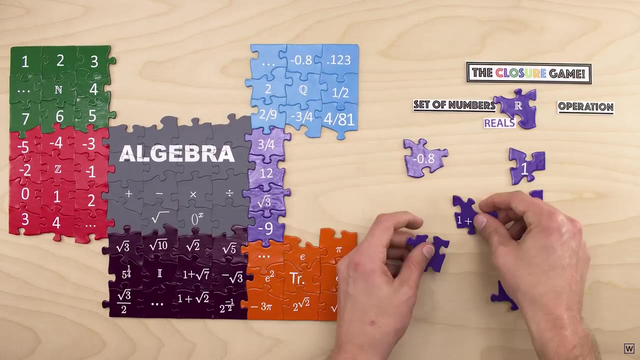 numbers like pi and e. We'll also save these for another day. So we've expanded our number system again to include irrationals, and all these numbers taken together form what we call the real numbers. Let's play our game one more time. Our set is now the real numbers and our operation. 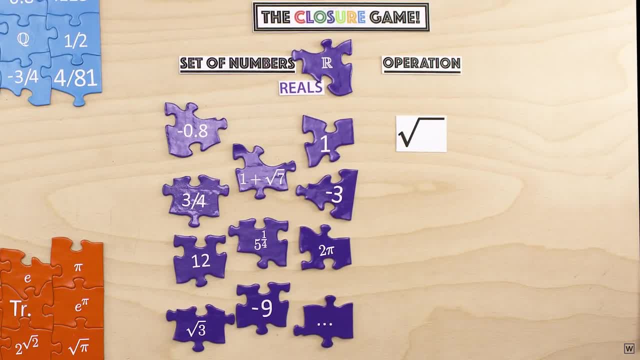 is taking roots. Do we have closure? Are there any real numbers that, when we take some root, we can yield a result that is not a real number? The answer is that, despite all the types of numbers we've included along the way, we're. 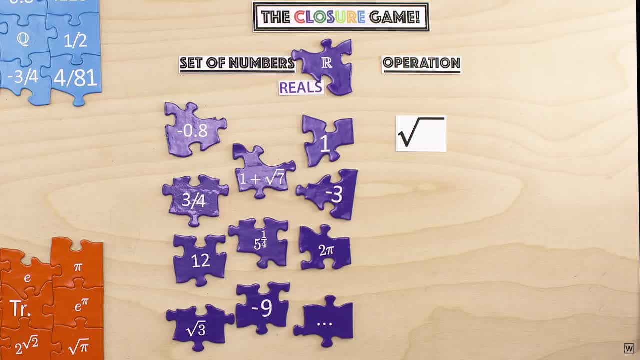 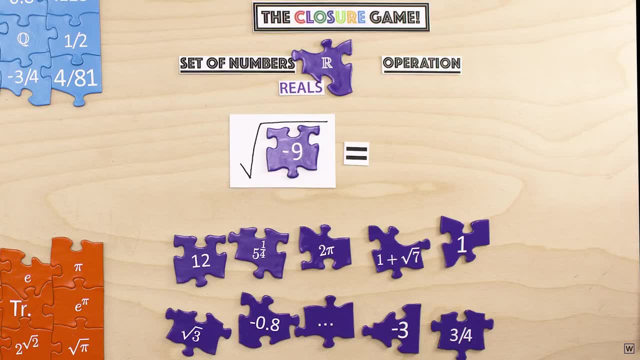 still missing something. We can write an expression only using real numbers and roots, for example the square root of negative 9,. that has no solution in the real numbers. For this problem to have an answer, we must expand our number system once more to include 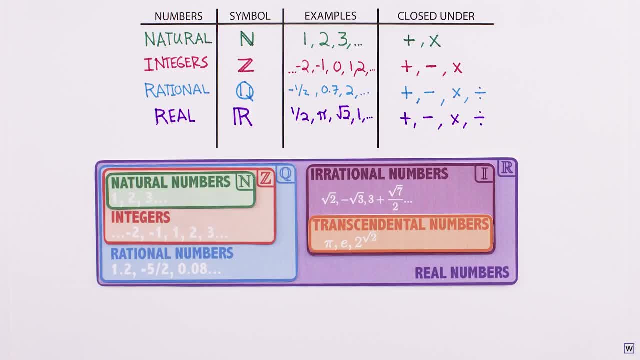 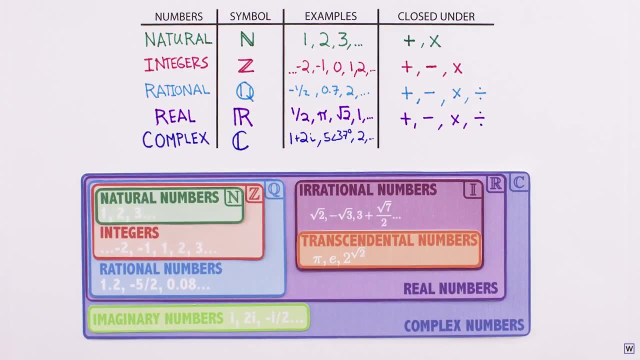 imaginary numbers And taking all our real numbers from before together with imaginary numbers, we arrive at our broadest class of numbers, That's the real numbers. We have to take root of the real numbers, the complex numbers. Initially, mathematicians were concerned that even complex numbers were not sufficient. 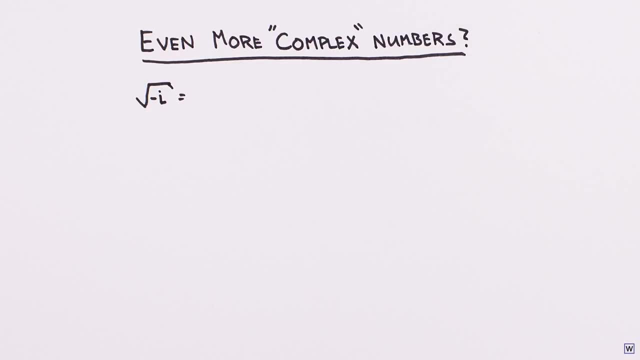 That problems like the square root of negative i would result in an even more complex number, Perhaps even a three-dimensional number, instead of our two-dimensional complex numbers. Fortunately, this turned out not to be the case. In fact, we can evaluate the square root of negative i, again using our good friend, the complex plane. 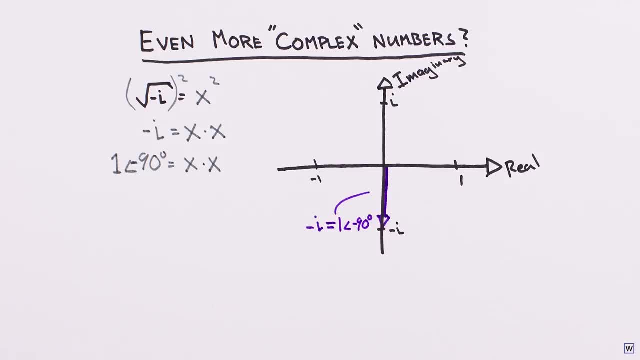 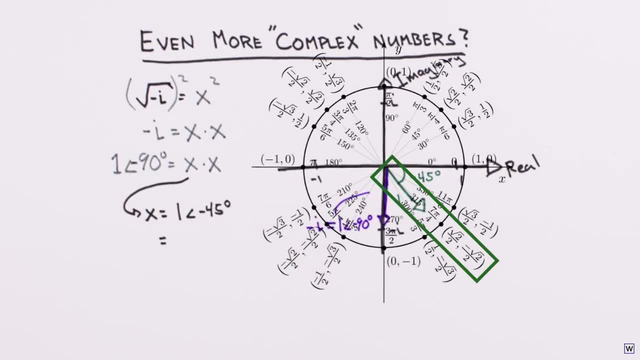 Since negative i has a magnitude of 1 and an angle of negative 90 degrees, we just need a number with a magnitude of 1 and an angle of negative 45 degrees, according to our unit circle, root 2 over 2 minus root 2 over 2i. 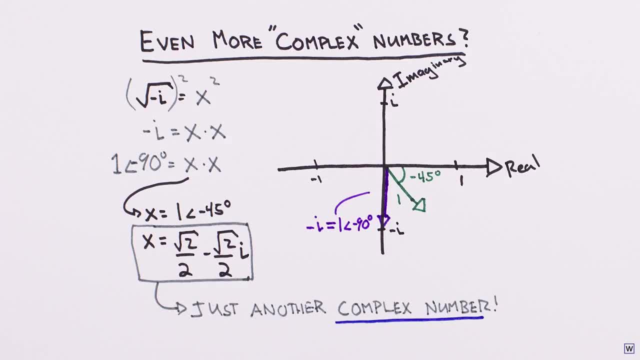 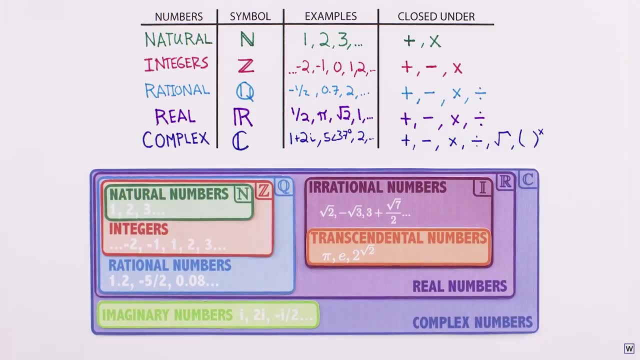 So the square root of negative i is just another complex number. There's no need for some wild new three-dimensional number. In fact, there's no operation in the world using addition, subtraction, multiplication, division, powers and roots that the complex numbers can't handle. Imaginary numbers are.